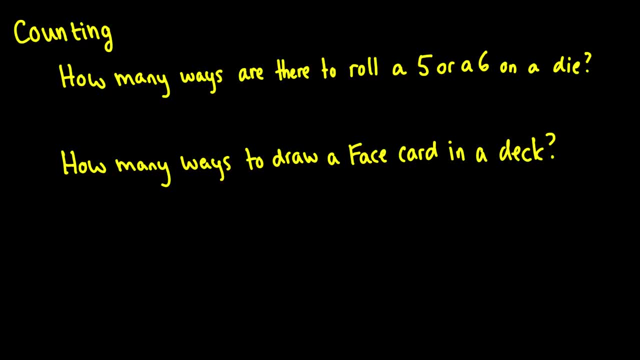 point of learning how to count is not about learning formulas. it's about learning how to abstract what you're trying to figure out and then applying a formula. Since a lot of these questions, knowing the formulas will get you 20-25% Knowing how to apply the formulas. 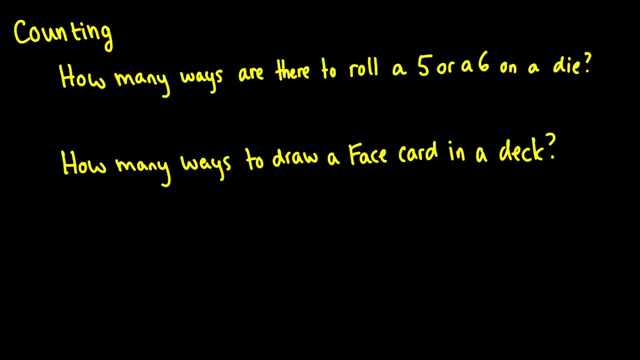 and how to figure out what the problem is. asking is, what separates the A's from the B's and C's? So let's start off with some intuitive things. How many ways can you roll a 5 or a 6 on a die with 6 faces? I assume all dice are 6-sided dice and all decks are. 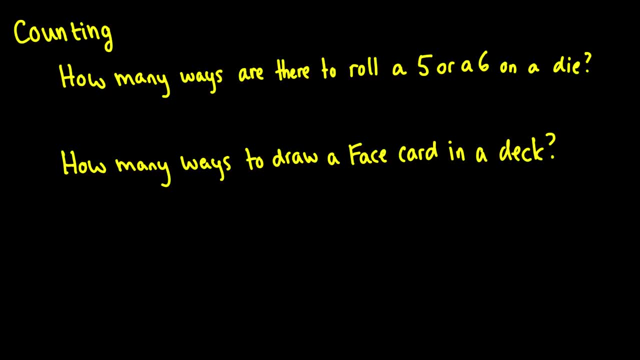 52-card decks without faces. How many ways can you roll a 5 or a 6 on a die with 6 faces? I assume all games are decided based on the number of faces, so it's kind of a doubt. jokers, These are the assumptions that I'm making in all of the questions. So how many ways? 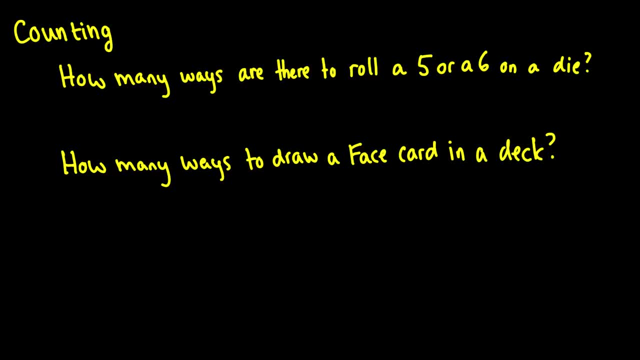 can you roll a 5 or a 6 on a die? Well, it's pretty easy. There are two ways. The possible ways that you can roll are one, two, three, four, five and six. So you can roll a 5 one. 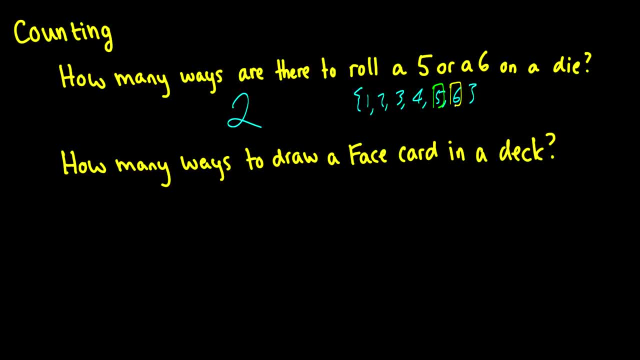 way and you can roll a 6 the other way, and therefore the answer is 2.. How many ways can you draw a face card in a deck? face cards are jacks, queens and kings and you have diamonds for each of them. you have clubs for each of them. my terrible drawing of clubs, that's not. 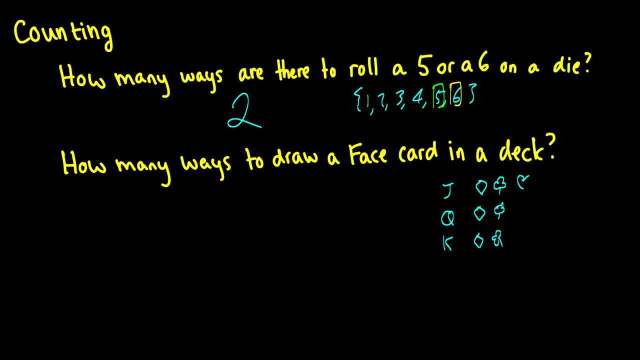 even a club. that's so terrible. you have hearts for each option and you have spades for each option which, surprisingly, my spades look much nicer. so here you can see that there's 12 possible ways to draw a face card as your first card. of course, if you drew a second card, you would have less ways. 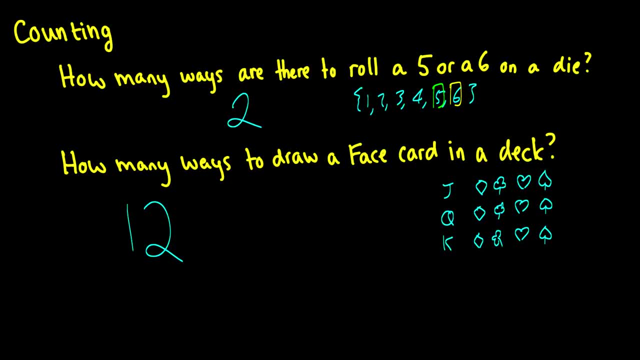 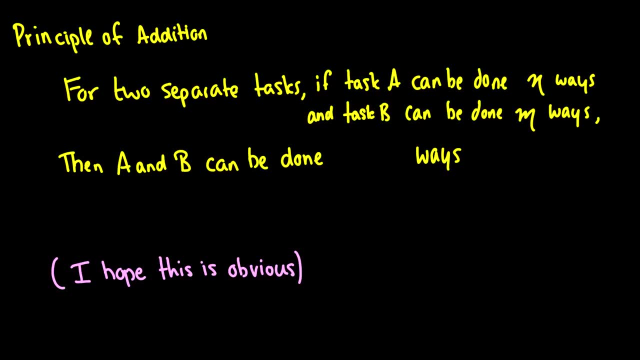 because you just took one out, but what we have there is an example of the principle of addition. so what we say is, if we have two separate tasks- a and B- and a can be done- you can draw a face card- and a can be done in n ways and B can be done in m ways. of course, these are variable numbers, then. 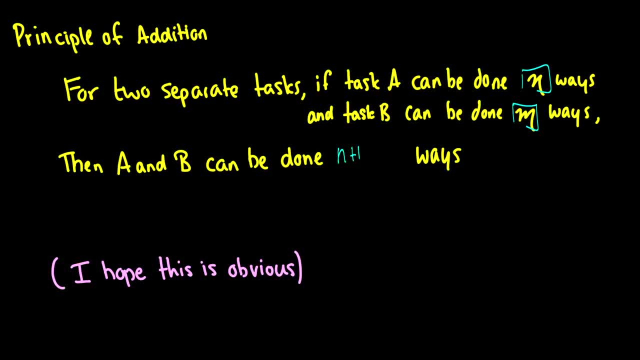 both of them together can be done in n plus m ways. I really hope this is obvious. for instance, how many ways are there are there to roll a 5 or a 6 on a die? there's two. how many ways are there to draw a face card? there's 12. how many? 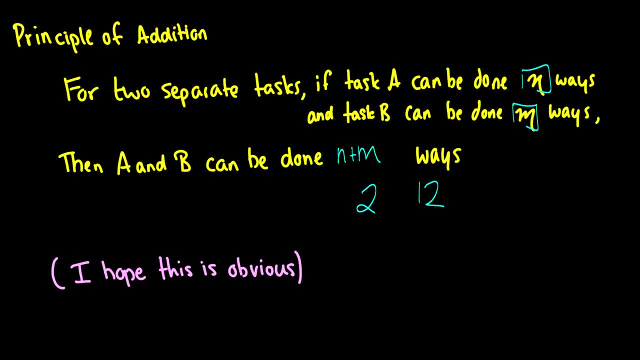 ways are there if I want to roll a die or draw a face card. so if I say, okay, I want a 5, 6 or a face card, or is a very, very key word, in fact, I'm going to write it in capital letters: I'm 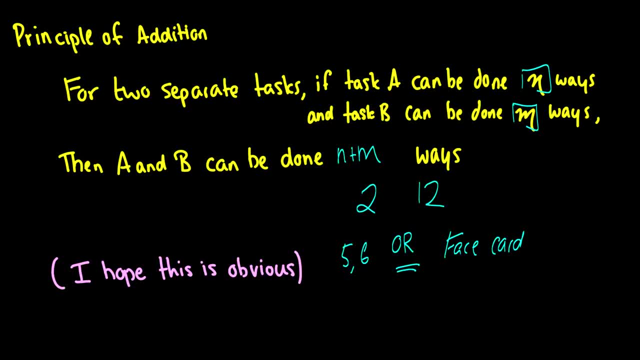 going to make the R look like a nice R. this is the same thing as 2 plus 12, which is equal to 14. the word or usually means plus in these sort of scenarios. this is not always okay. this is not always so when I say these things. 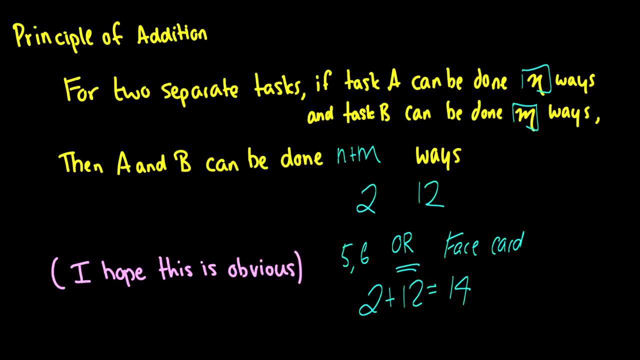 this does not mean always. this means likely. you have to read the question and you have to think: what are they asking? that is the most important part is to ask yourself what is the question asking of you, because the words will not always directly translate into formulas. you have to abstract what they're saying and 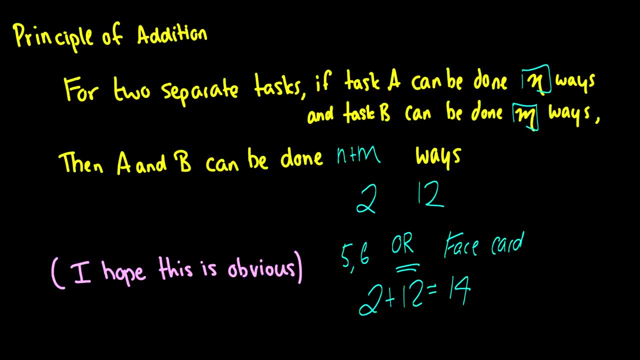 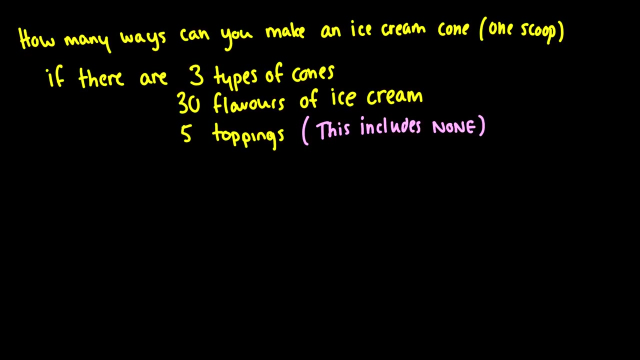 turn it into a scenario in your head and then figure out what to do next, and then directors of A papier or negotiated what to do from there. so if I say 5 or six or a face card, that's task, one task. to put them together, you get 2 plus 12, which is 14. there's 14 ways to roll up 5 or 6 or draw. 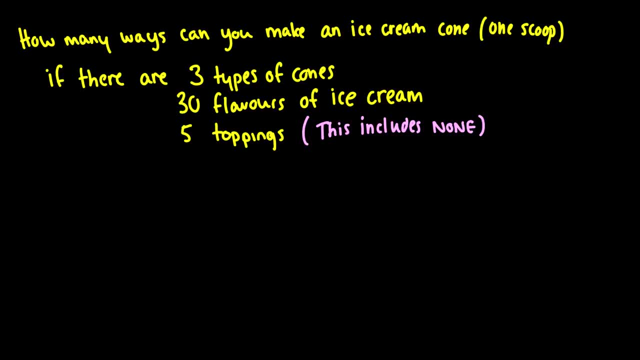 a face card, okay, of ice cream and five toppings, But we're really going to say there's four toppings and one of your options is to have no toppings. So we're going to say it's five toppings. Well, first of all, step one is you need to pick a cone. So 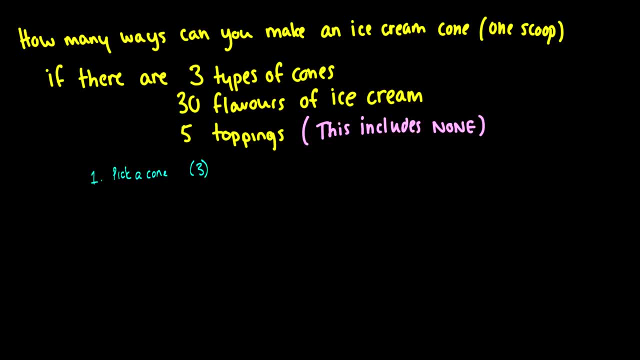 there's three possible ways you can do: the first one And then your second one. you need to pick a flavor. So, if you have nothing, your first choice is going to be one of three cones. Your second choice: you're going to have 30 different. 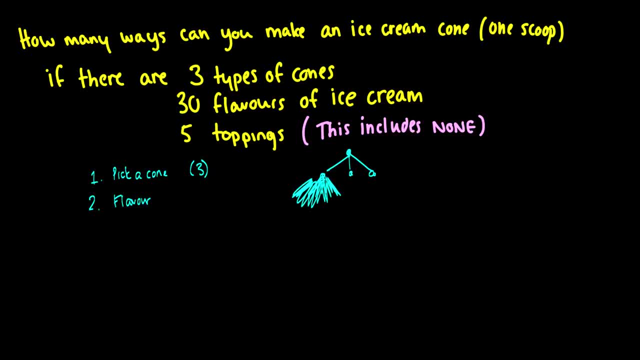 flavors to choose from. So this is a very terrible tree to draw, but each option has 30 there, And then your last one- you have to pick a topping, and each one of these three choices will have a fill Tball. Now, if you were asked to draw a, 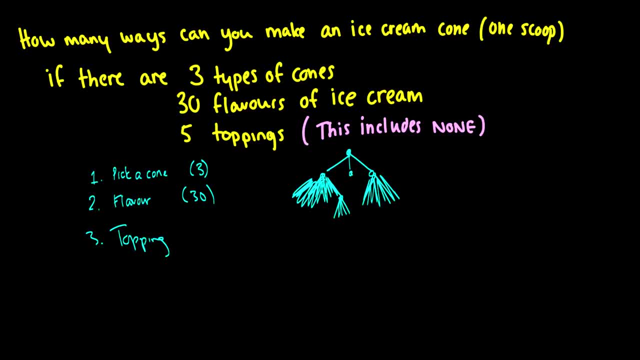 these little nodes here is going to split off into five different parts because you have five different options. So the total number of ways to do this is going to be 3 times 30 times 5, which is 450 ways. Now, why is this? Well, because there's 30 different flavors of ice cream. 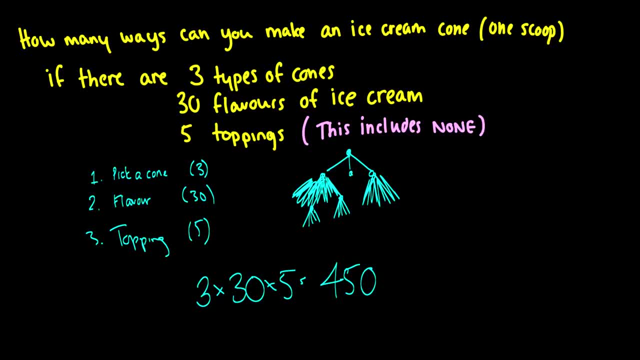 and each one of them can be matched with one different type of cone. So you can have 3 times 30 combinations of cones and ice cream. So you have 90 different ice creams. And now you take each one of those ice cream and you say, okay, which one of these five toppings do I want on it? 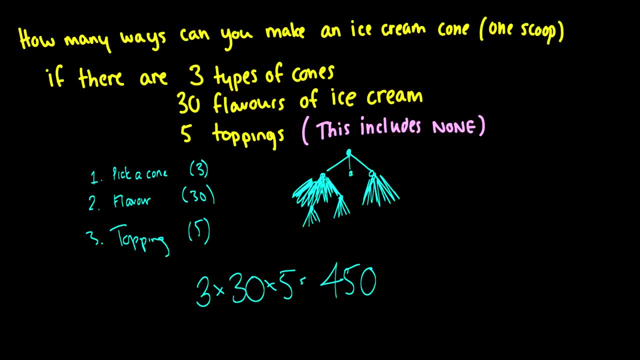 So you have 90 times 5 different topping options. So that's 450 total different types of ice cream you can get with only three types of cones, 30 flavors and five toppings. So you could bring 450 people and everyone could get a different ice cream cone- Somebody. 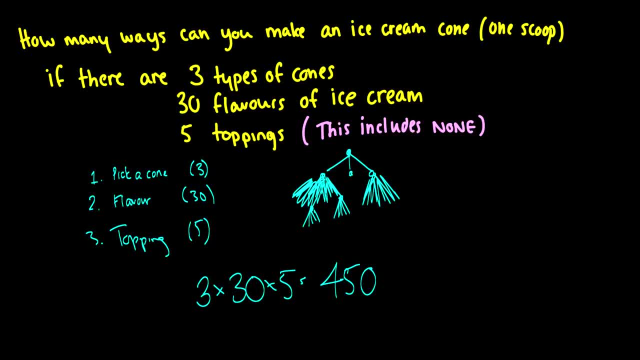 of course, would end up with like prunes with gummy worms and like a sugar cone. So I mean those poor, poor souls, But in the case that that exists, I mean someone can have it right We. 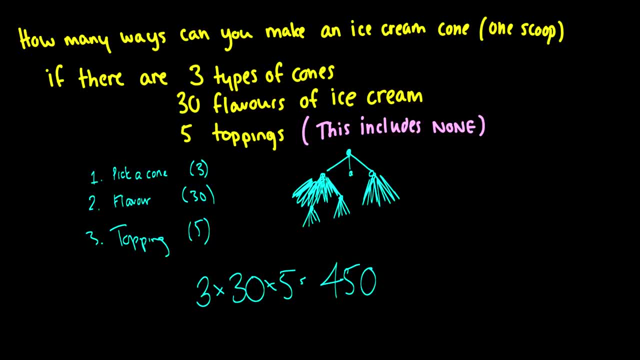 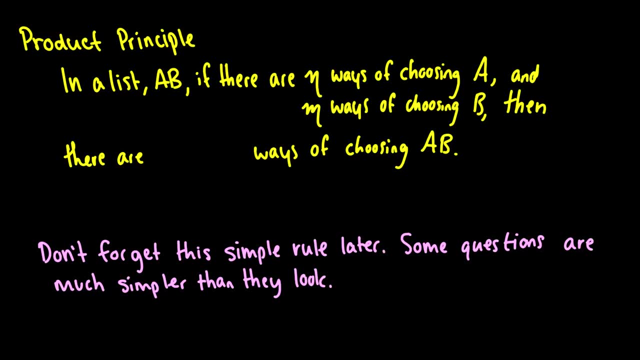 can't just count the good flavors, because then there would only be like 16 possibilities. We have to count all of them. Anyways, this is called the Product Principle or Principle of Multiplication, And we say in a list or a set of tasks, A, B, 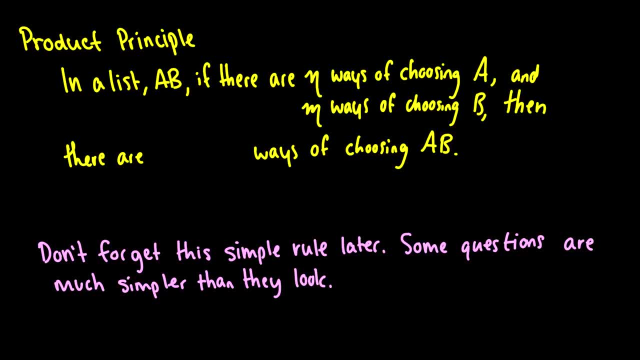 if there's n ways of choosing A and m ways of choosing B, then there are n times m ways of choosing A- B And basically these are subsequent tasks, or subsequent tasks, which means we do A, then we do B, then we do C, and this occurs in a list. 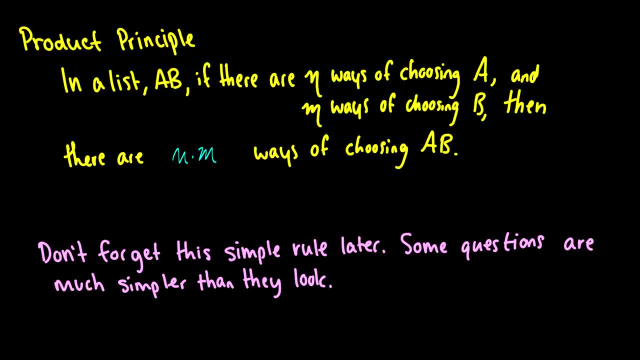 And what I will want to say is that these rules of products and addition are very primitive. You're going to find very difficult questions later. Do not forget these basic principles because sometimes a very difficult looking question can just be a very simple application of the product or addition principle. 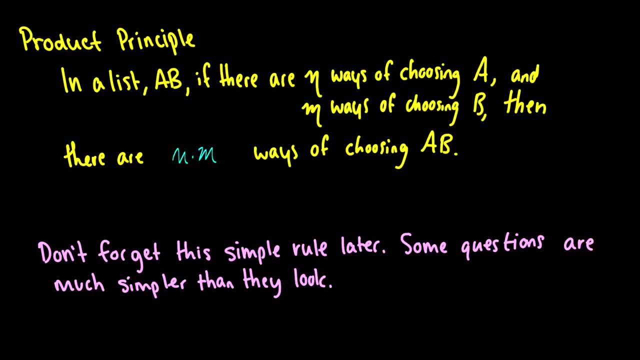 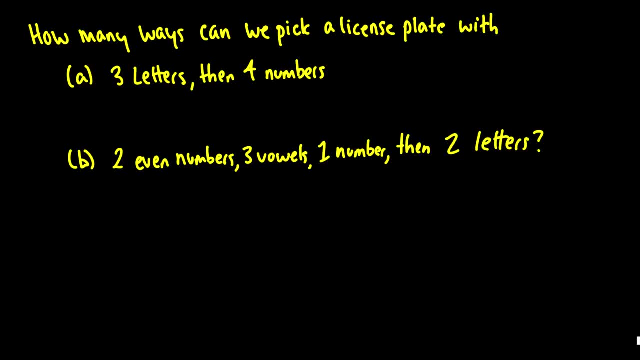 So please remember these. But let's do an example here with license plates. Every textbook loves license plates and I love license plates as a first example. So how many ways can we pick a license plate that has three letters and then four numbers? I'm going to go through the step-by-step. 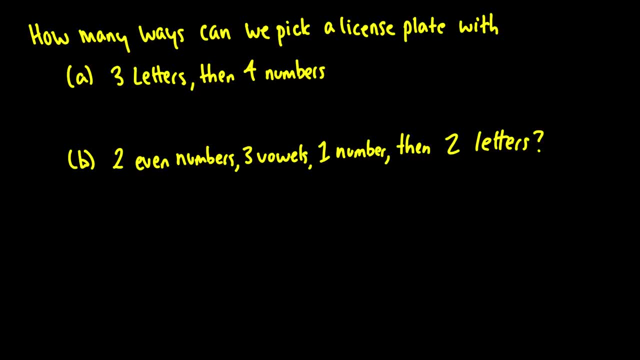 process with you. and let's think about this: It's not saying that letters cannot be repeated. So how many letters are there in the alphabet? Well, there's 26.. So the first letter has 26 options And then the second letter has 26 options. So we want to multiply because we can have 26 times. 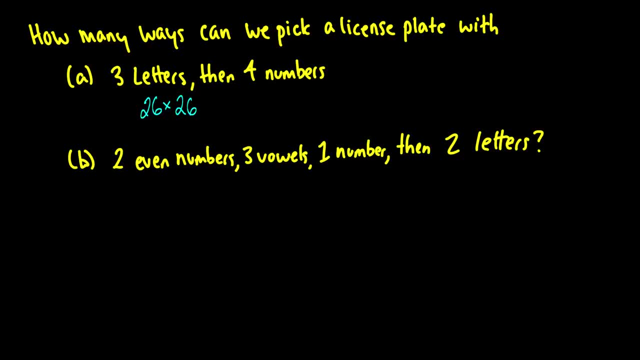 26 combinations of two letters. Okay, and now the third letter has 26 options. Now we move on to numbers. There are 10 numbers: 0, 1,, 2, 3,, 4, 5, 6,, 7,, 8, 9.. So we have 10 numbers for the first number. 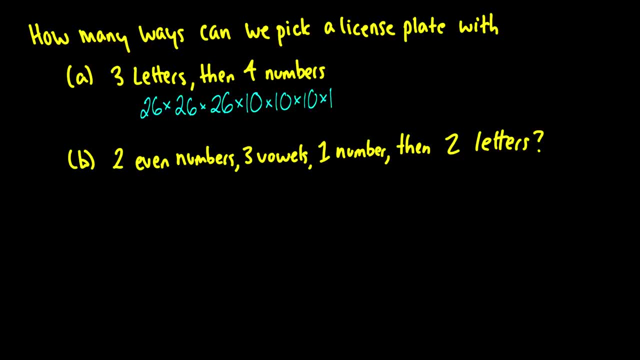 We have 10 numbers for the second, third and fourth. So we have this number here, which I'm going to shorten to 26 cubed times 10 to the 4, and that is how many options you have for a three-letter, four-number license plate, So you're not running out of license. 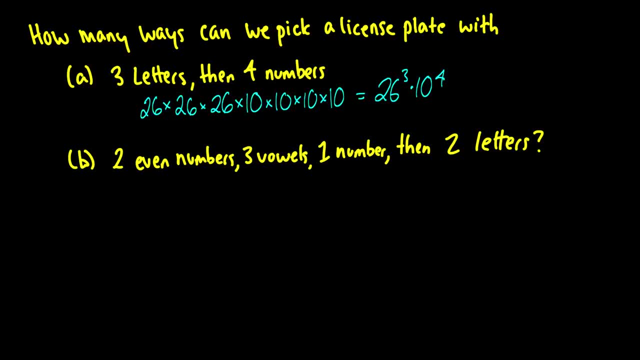 plate numbers anytime soon. What if we were a little bit more specific and we want a license plate that looks like 42AEO6GH? What if we want a license plate to look like this? Well, we want even numbers. So how many? 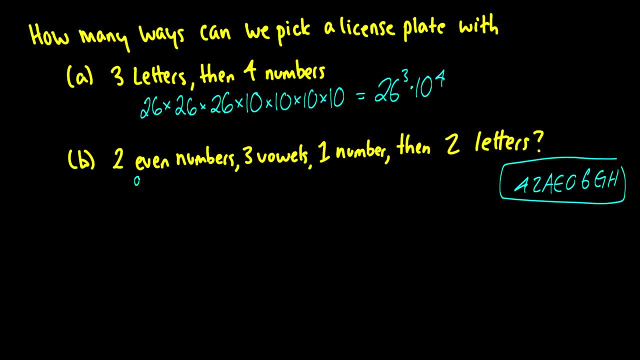 even numbers are there. Well, there's 0,, 2,, 4,, 6,, 8.. So we have five to choose from for the first and second. How many vowels are there? Well, there's A, E, I, O, N, U, sometimes Y, sometimes W.